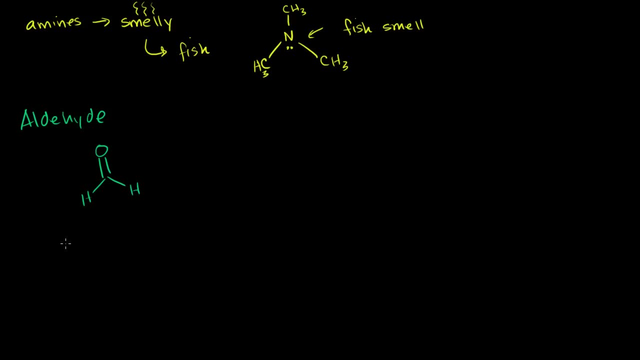 So this right here is formaldehyde, and that's the common name, And you've probably seen it used as a kind of a preservative, maybe even in your biology class. if there's like a dead frog in a solution, it's probably inside. 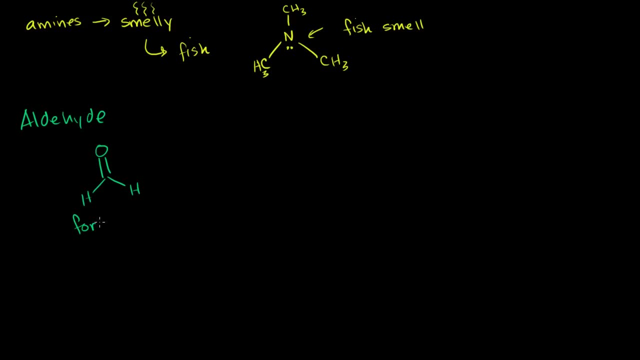 of formaldehyde. Let me write this down Once again: this is the common name. I'm going to teach you in a second how to systematically name these things. But when you have larger aldehydes, they actually can have a pretty sweet or even a rosy smell. 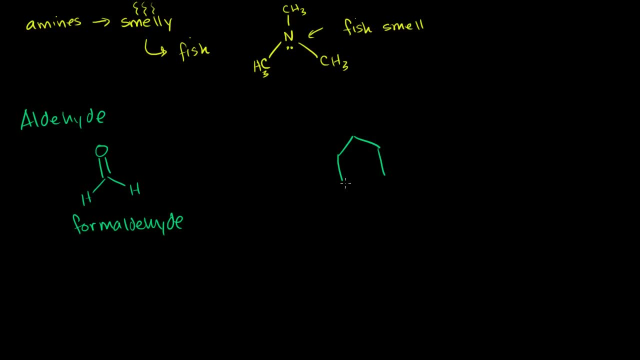 So you have something like benzaldehyde, which you actually saw when we started the benzene derivatives. So this is benzaldehyde, right over here, This molecule. let me write this down: This is benzaldehyde, And then this molecule here, just when I tell you what it's. 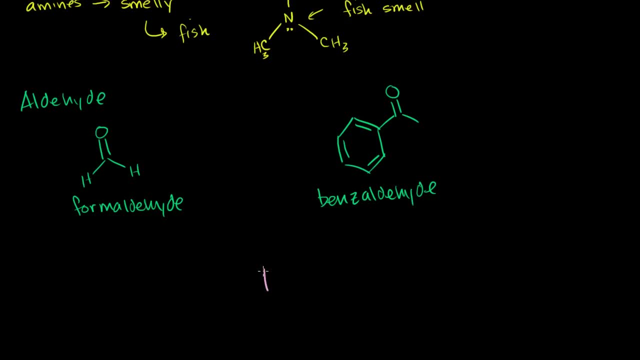 called. you'll probably guess what it smells like. So this has a benzene ring. You have a benzene ring like this, And then you have one, two, three carbons, The last one's double bonded to an oxygen, and then a. 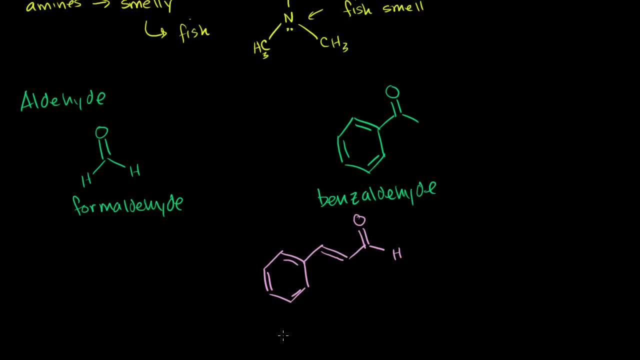 hydrogen, Hydrogen like there- And they have a double bond right over here And this is called cinnamaldehyde And, as you could guess, this smells like cinnamon And in fact, this is the molecule in cinnamon that gives it its smell, although you don't want to have large. 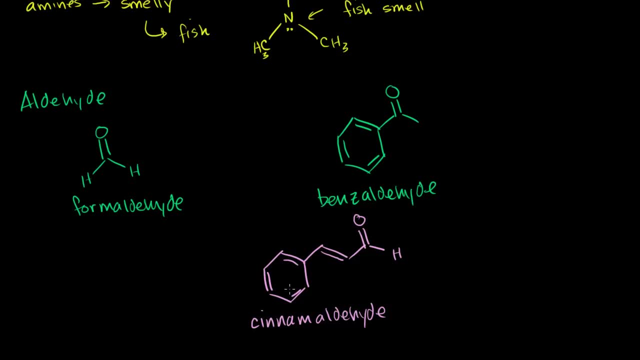 quantities of it or it might be poisonous, But in cinnamon it's a very pleasant thing. So larger aldehydes tend to have kind of a nice rosy, sweet, flowery smell. Smaller ones tend to be kind of pungent. 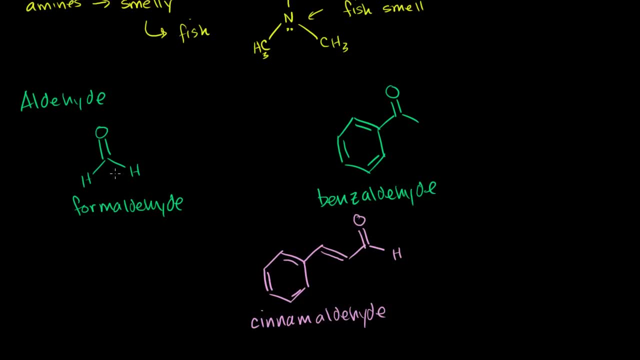 If you open up that jar in your biology class and smell that frog, it will not be a pleasant smell. So now that I've talked about smell enough, I think let's talk about what makes an aldehyde an aldehyde, And you might even see a pattern here. 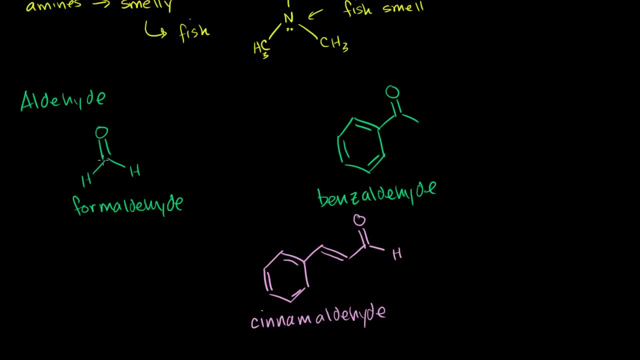 In all of these aldehydes that I've drawn, we have a carbon double bonded to an oxygen, Carbon double bonded to an oxygen, And actually this part of it right here, And we'll see this over and over again- This is called a carbonyl group. 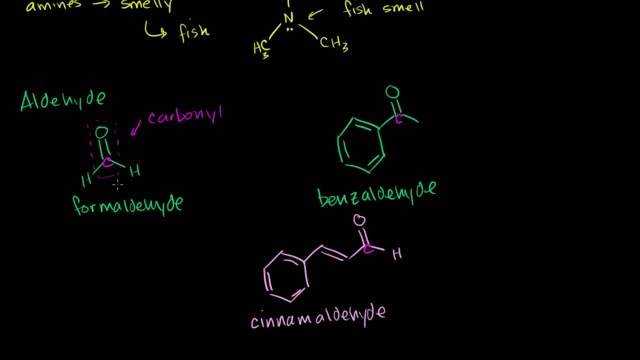 So that is a carbonyl group. This right here is a carbonyl group And you even see it over here. But that by itself is not the distinctive feature of an aldehyde. You'll see that in other types of molecules. 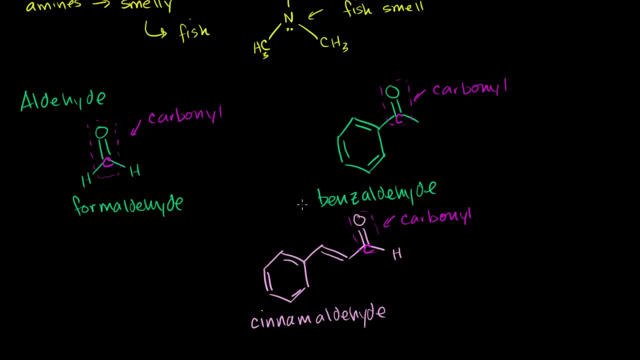 Let me write it here: Carbonyl. What's distinctive about an aldehyde is attached to the carbon in the carbonyl. You have a hydrogen, here You have a- and I'm sorry I forgot to draw this hydrogen here. on benzaldehyde: 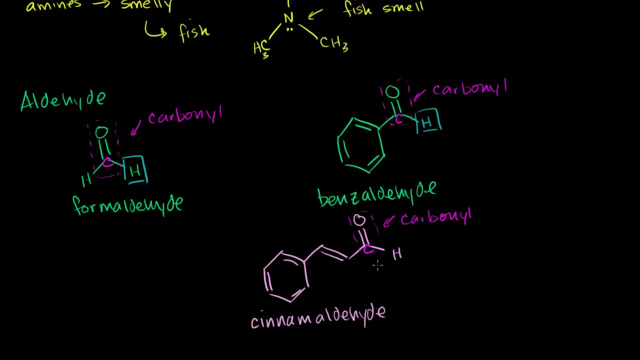 You have a hydrogen here, You have a hydrogen here, You have a hydrogen here. So in general, an aldehyde is something that looks like this: You have a carbonyl group, You have a hydrogen, And then you just have some other type of carbon chain. 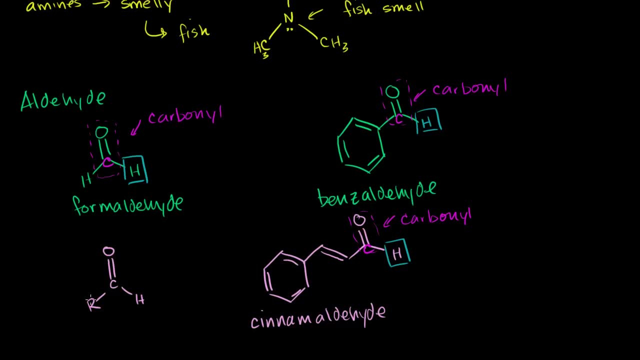 This right here is the simplest possible aldehyde, And actually this chain ends up being just another hydrogen. Now, these three that I've shown you right here, these are their common names And these are the way that most people will talk about. 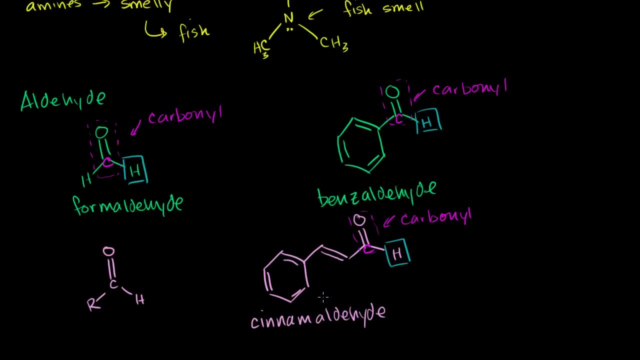 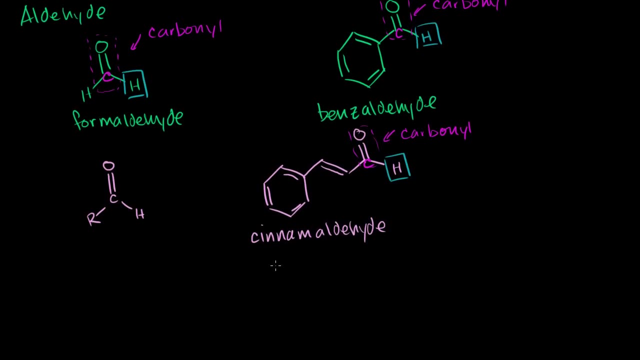 formaldehyde, benzaldehyde or cinnamaldehyde. So they're just kind of good to know And I'll show you one more. This is a pretty important one. Let me do it down here so we have some space. 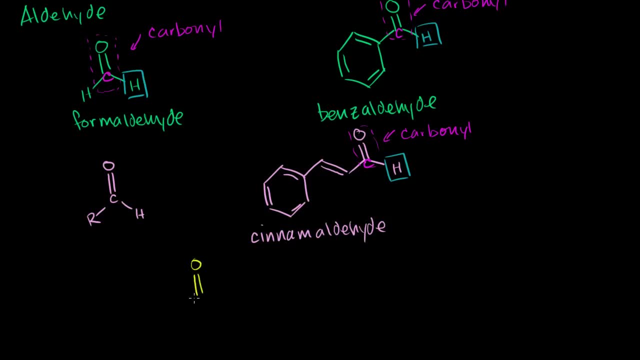 So another one looks like this, So bonded to a CH3 over here, And then a hydrogen, And this right here is called acetylaldehyde, And I just wanted to expose you to these common names because this is what people normally use for these molecules. 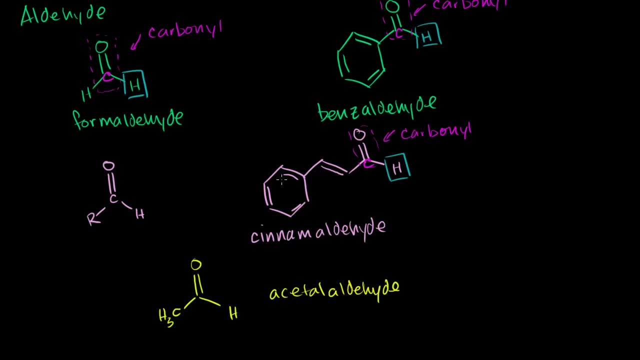 Now there is an IAPUC. I always forget the acronym. There is a systematic way to name them And it's actually pretty straightforward. You just look at the longest carbon gene And you always start numbering at the carbon that's in the carbonyl group. 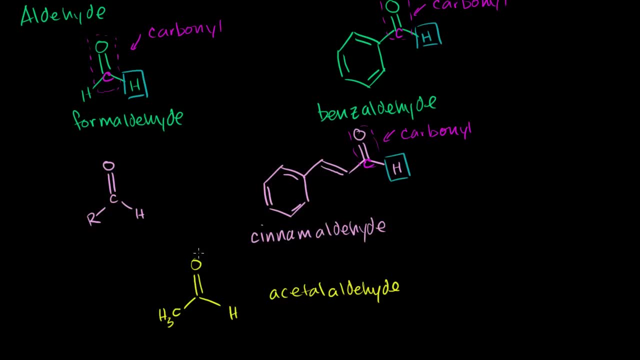 And it's always going to be at the end of the chain, because that's always going to be bonded to a hydrogen. And actually let me just make clear that this is also an aldehyde. You have your carbonyl group And on one end you have a hydrogen, just like that. 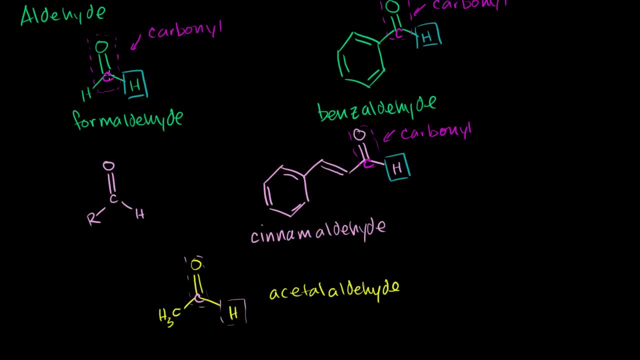 Now the systematic way of it. you just look at the longest carbon chain Over here. there's just one carbon. So here you would call this the systematic name. You would call this methanal, not methanol. Methanol means you would have an OH group. 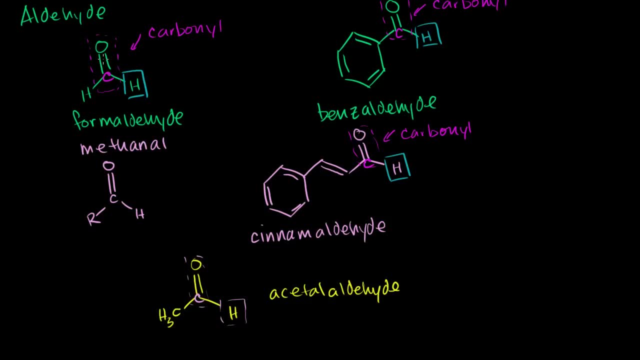 But since you have this double bond and you have a hydrogen, or you could say, this double bond is at the end of the carbon chain. this is an aldehyde, So the systematic name is methanol, not methanol. Let me make that clear. 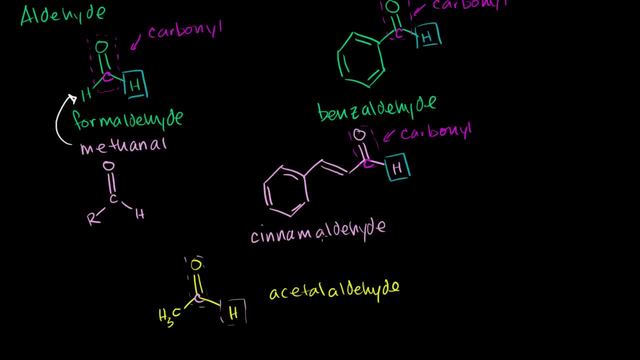 This is methanol, right there, This one. I won't do cinnamaldehyde or benzaldehyde, because this is really the only way that people name it. Actually, frankly, formaldehyde, people never call it methanol And acetylaldehyde: they'll never. 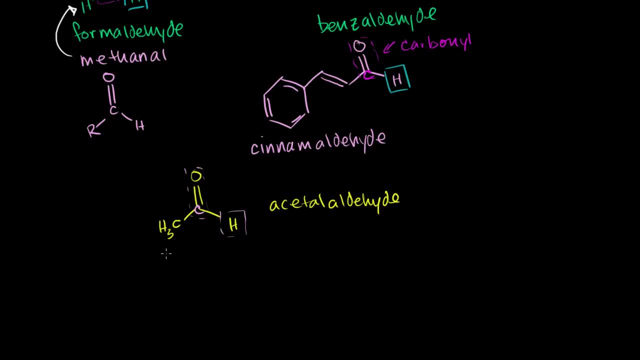 call it what I'm about to name it, But the systematic name is the longest carbon chain. You have one, two carbons, So it is ethanol. I don't want to pronounce it incorrectly. Let's do a couple more of these just. 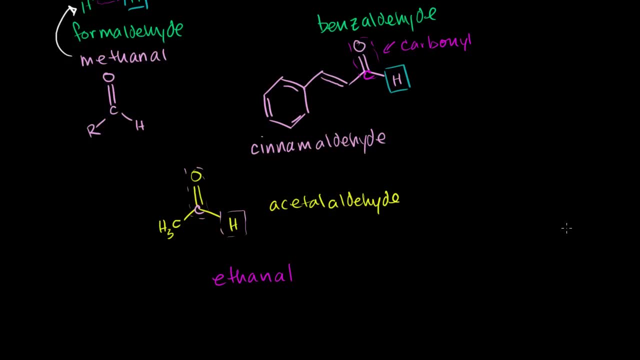 to make sure we have a decent understanding of the systematic names here. So if we were to name- and in general, if you have a really long chain, the systematic names are what is used. So this thing right here, what would you call it? 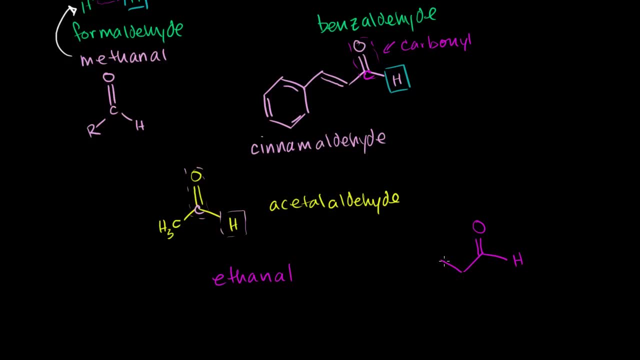 It's clearly an aldehyde. You have a carbonyl group, a hydrogen, And you have one, two, three carbons. So three carbons. the prefix is prop, So it's propanal, It's an aldehyde. 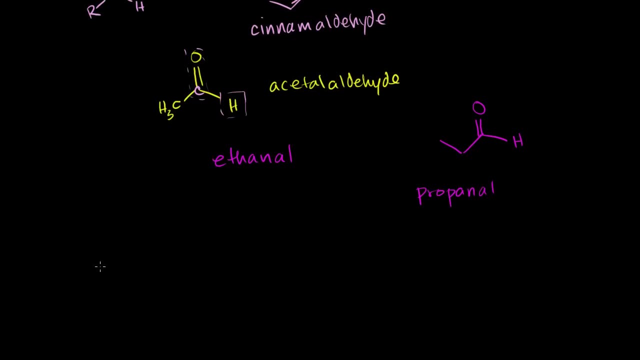 If we want to do something slightly more complicated, let's do something like this. What would this be called? Let's see, We have one, two, three, four, five. We have five carbons. So it'll be a pent. 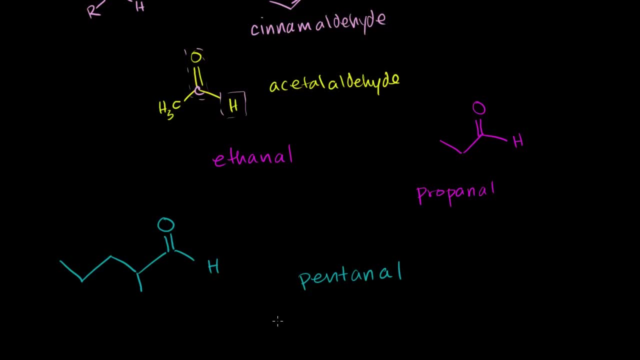 And then it's obviously an aldehyde, So it's pentanol. And you always assume that you start numbering at the carbon in the carbonyl group. So one, two, three, four, five, And on the two carbon you have a methyl group. 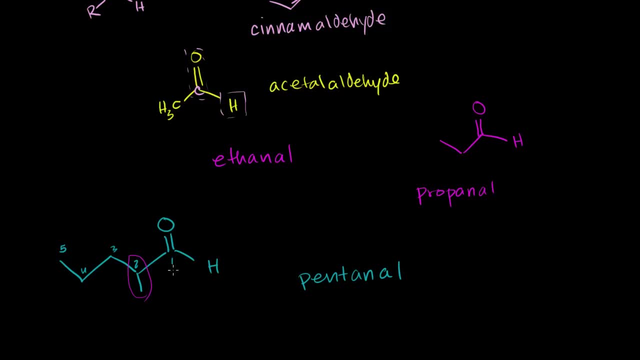 So this is 2-methyl, So you have a methyl group right here. So this is going to be 2-methylpentanol.